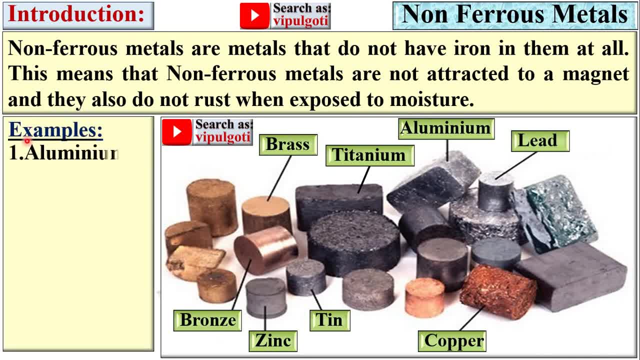 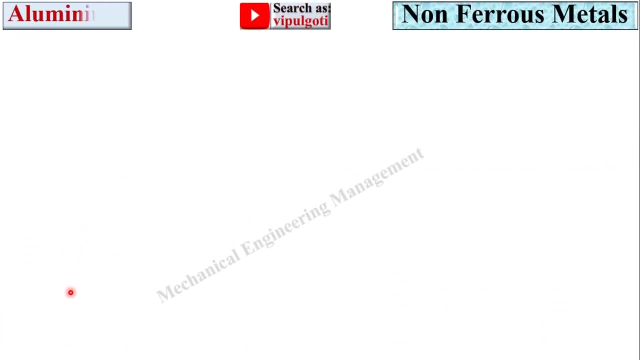 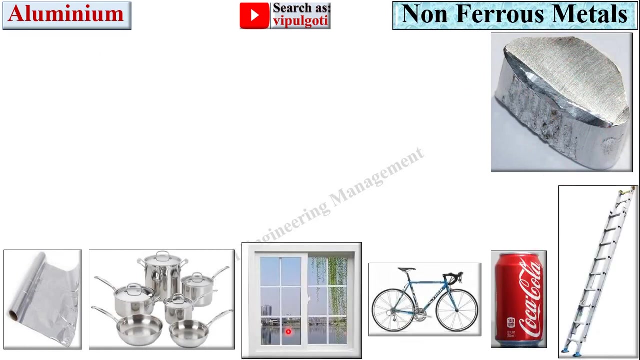 no, any corrosion. Examples of non-ferrous metals: aluminum, copper, zinc, tin, lead, nickel, titanium, silver, gold, etc. Now let's see one by one all the non-ferrous metals briefly. So first start with aluminum, and here you can see this is the aluminum and these are. 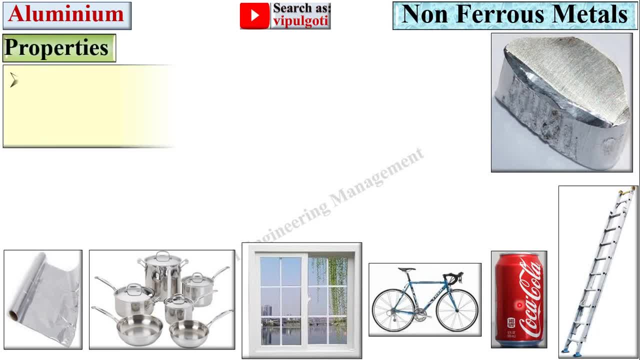 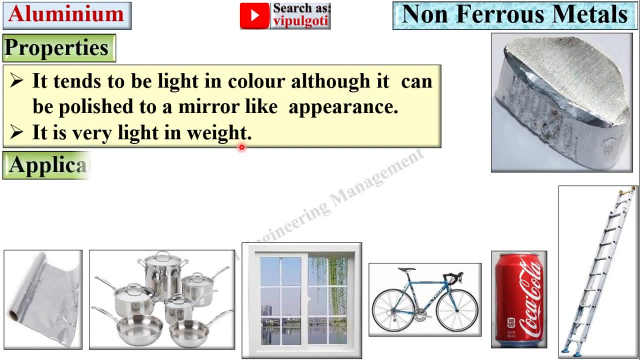 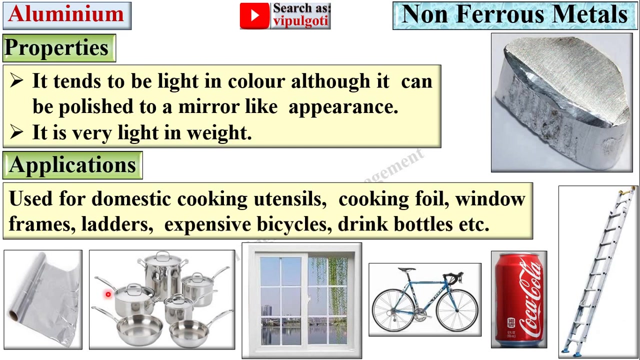 the different application of aluminum Properties. it tends to be light in color, although it can be polished to a mirror like appearance. It is very light in weight. Now applications used for domestic cooking utensils: Cooking foil- here you can see foil window frame cooking utensils, leather- expensive. 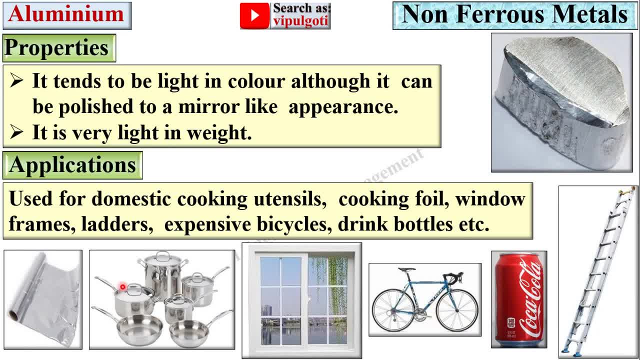 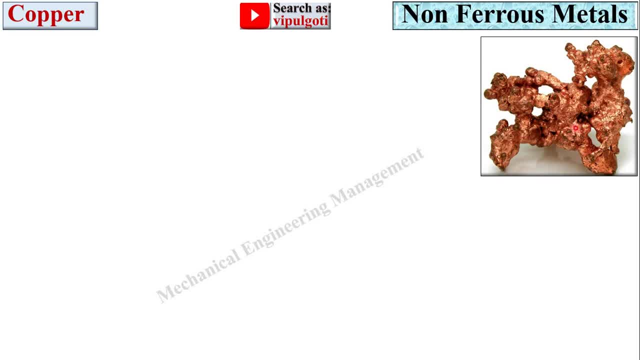 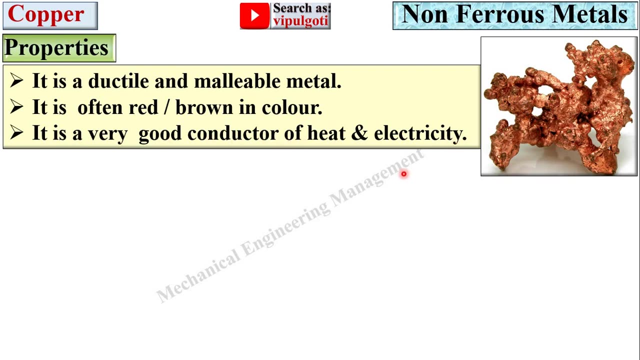 vehicles, drink bottles, etc. Now next copper, and here you can see copper Properties of copper, It is often red or black. It is often red or black, It is often brown in color. It is very good conductor of heat and electricity. 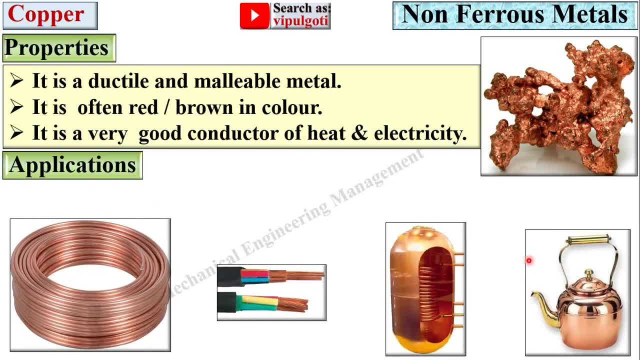 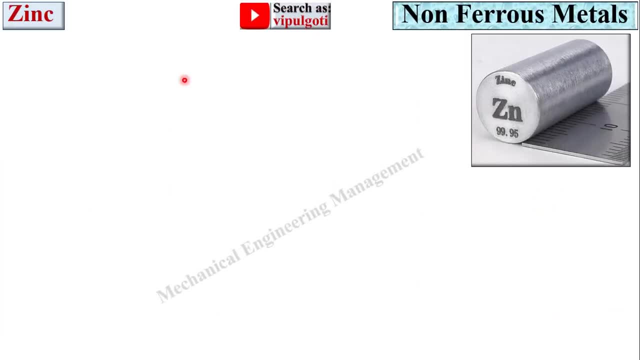 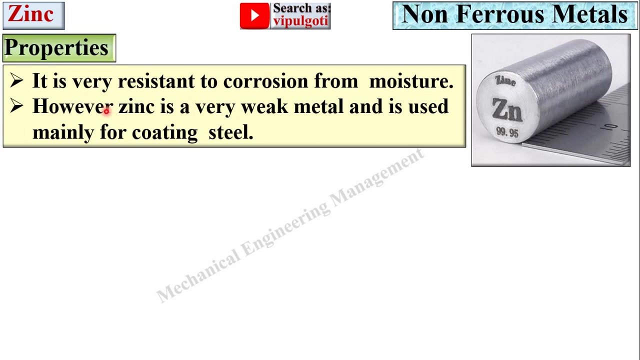 Now applications. So these are the different applications of copper: Used as tubes, electric wires, electric components, cook wires, etc. Next, zinc. Here you can see the specimen of zinc. Now let's start with properties of zinc. It is very resistant to corrosion from moisture. 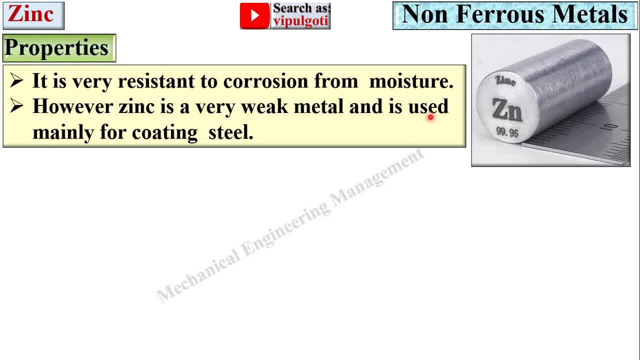 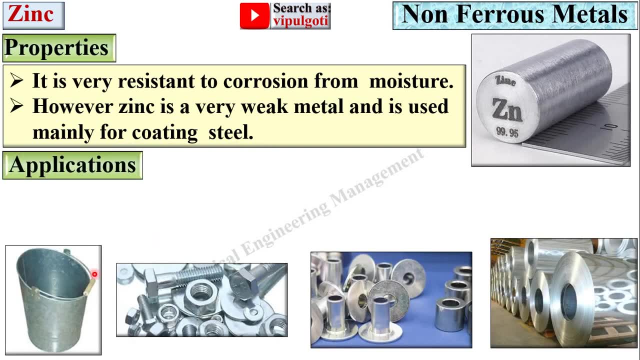 However, zinc is a very weak metal and is used mainly for coating steel applications. Here you can see Used as a coating on screws, steel buckets. It is also used to galvanize iron based metals, or you can say simply steel. Here you can see coating on the different material. 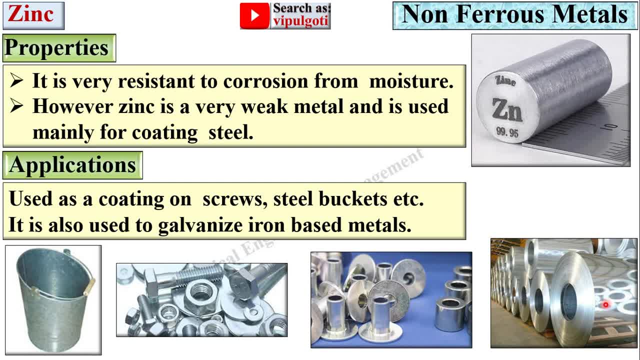 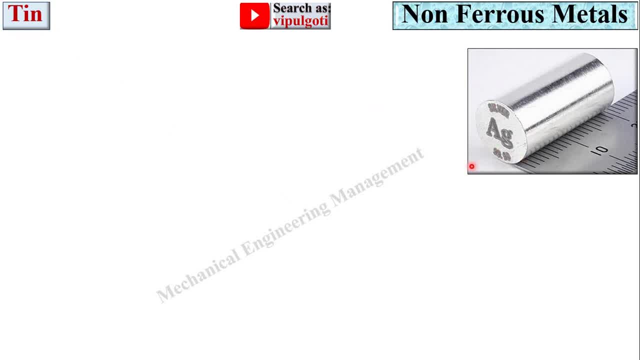 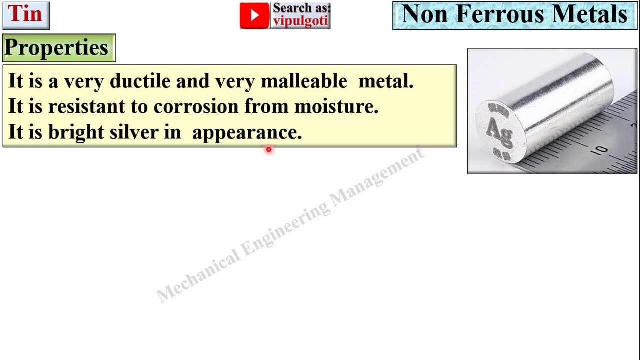 And here you can see the coating by zinc. Now it's turn for tin, and this is the specimen of tin. It is very ductile and very malleable metal. It is resistant To corrosion from moisture. It is bright silver in appearance. 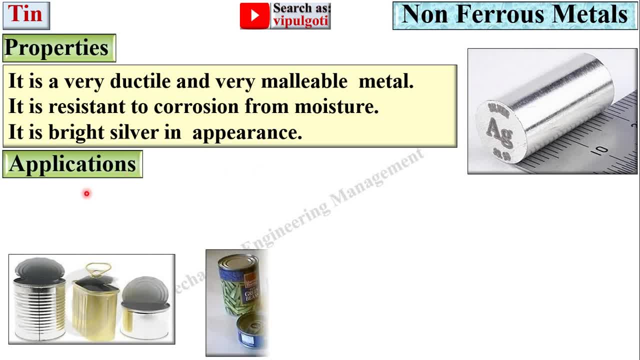 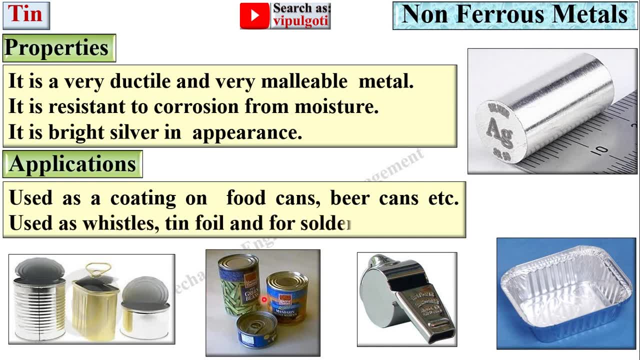 Here you can see bright silver. Now applications Used as a coating on food cans- Here you can see beer cans, etc. Used as vessels, tin foil and for soldering also. Now next, lead. Here you can see lead. It is soft and malleable metal. 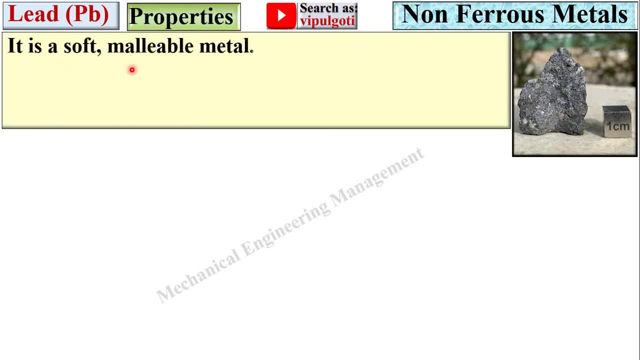 It is also counted as one of the heavy metals. Lead has a bluish white color- Here you can see- After being freshly cut, but it soon tarnishes to a dull grayish color when exposed to air. So when you cut it, 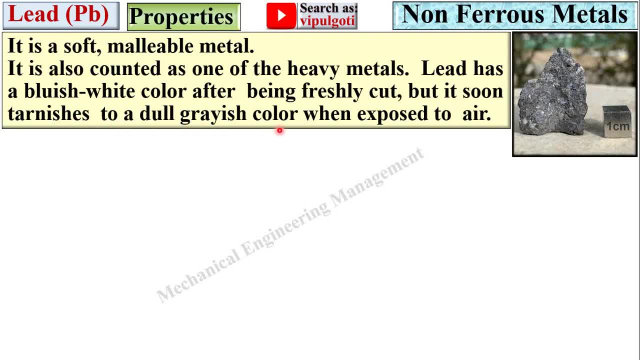 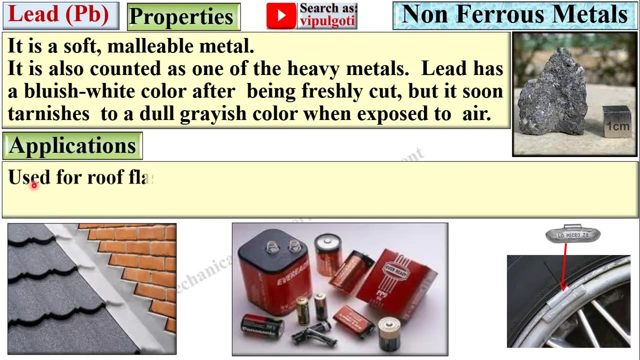 So initially it is soft and malleable metal, But when you cut it It is very thick. It is very light. Initially it is having bluish, white color and then soon it is converted into a dull grayish color. Now the applications used for roof flashing here you can see also used for batteries and 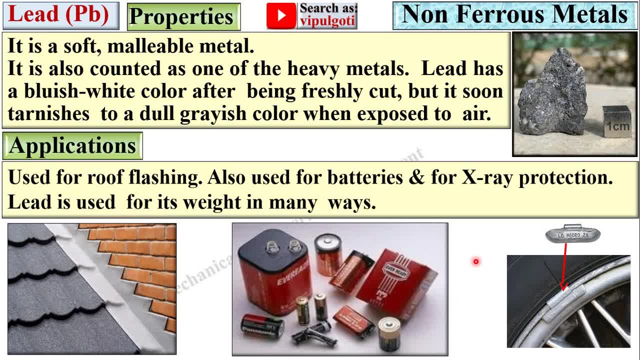 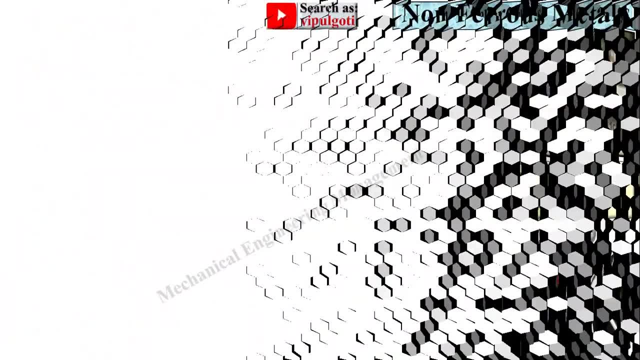 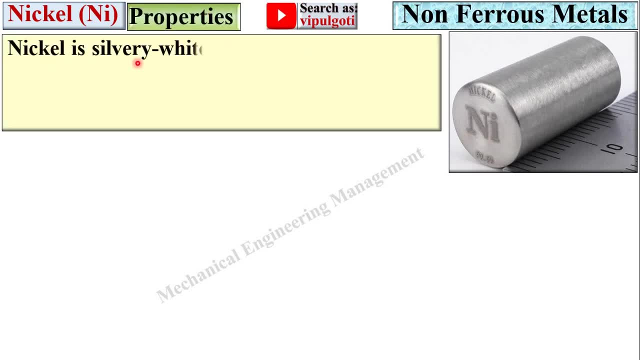 for x-ray protections. It is used for its weight in many ways- here you can see- because of it is heavy material. Now next, nickel. this is a specimen of nickel. Nickel is silverly, white, hard, malleable, ductile and magnetic in nature. 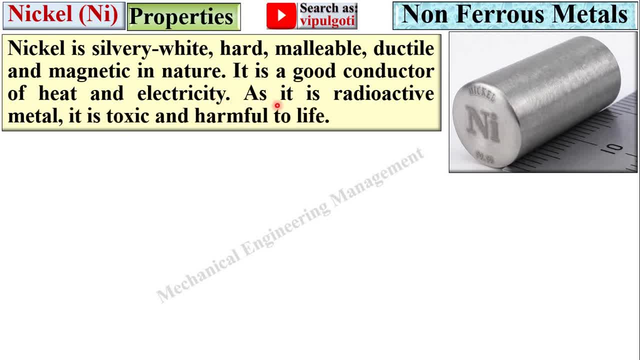 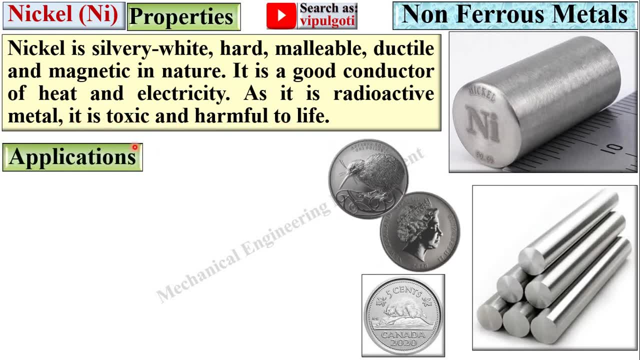 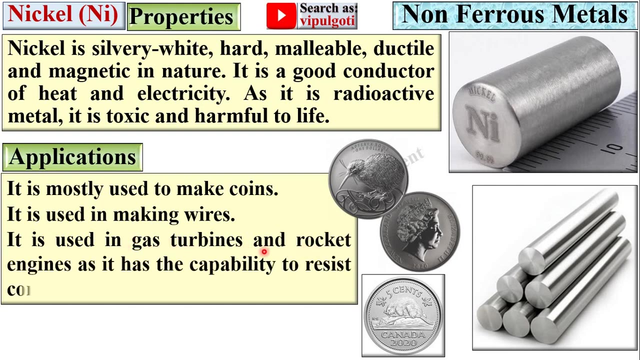 It is a good conductor of heat and electricity. as it is radioactive metal, It is toxic. It is toxic and harmful to life. These are different applications of nickel. It is mostly used to make coins. It is used in making wires. It is used in gas turbines and rocket engines, as it has the capability to resist corrosion.